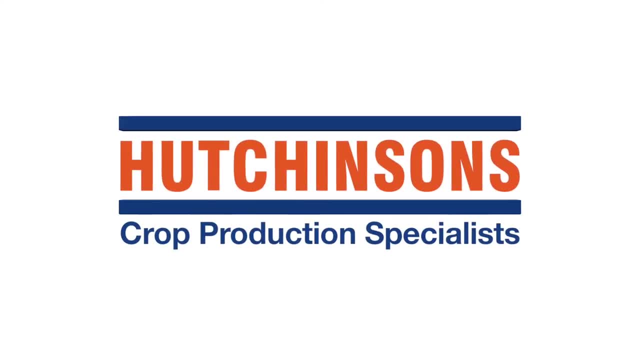 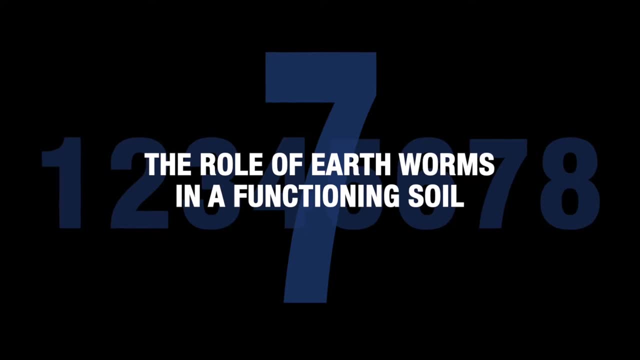 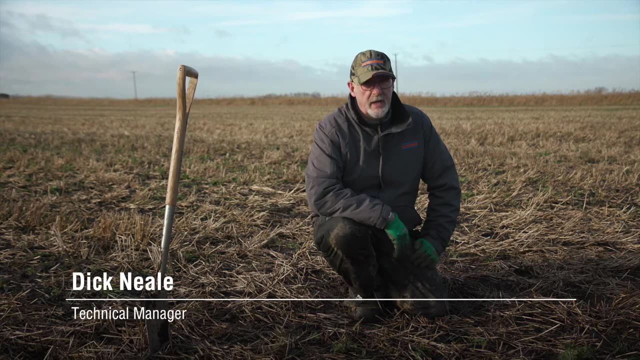 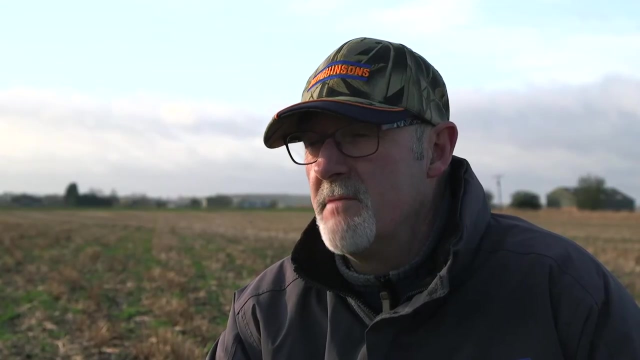 One of the most dominant features of healthy soils that we put more and more focus on, and particularly in recent years, with people like Jackie Stroud at Rothamsted giving us more and more information about earthworms and how they function and the types we should be looking for. 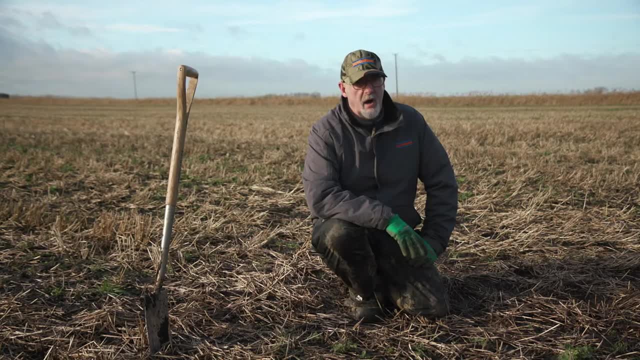 and how we should assess them. They really are a key part of healthy soil function. One of the issues with this soil when we started four years ago was we had no worm population. It was quite stark that they just were not here, and you cannot get really good soil function until you've got a. 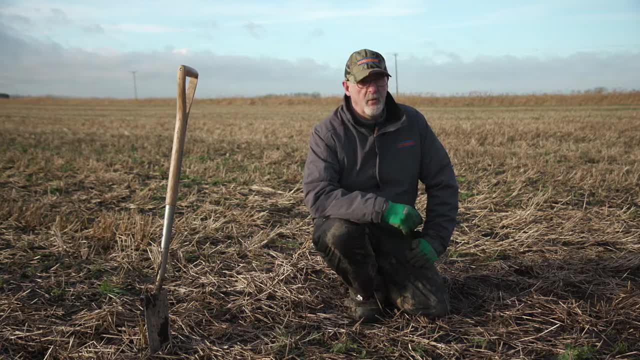 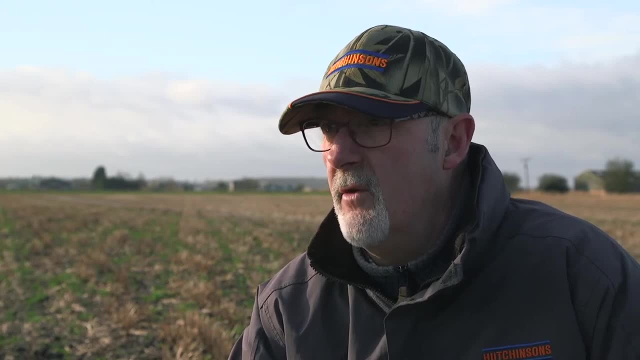 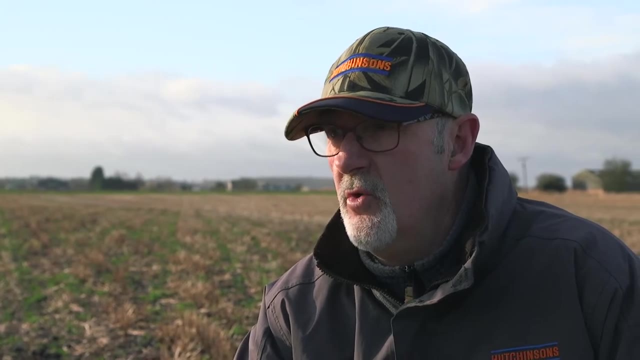 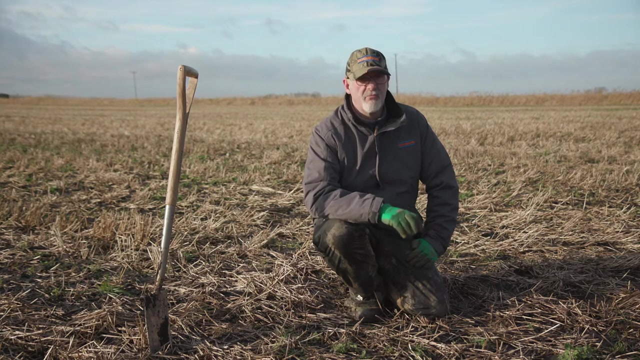 worm population built and helping you with drainage, with nutrient recycling and things like residue management from the surface of the soil, and also understanding that, depending on the species of worm that we're trying to encourage, we need to understand where they want their food source placed In the case of anisic worms, which is what we were really trying to build in these. 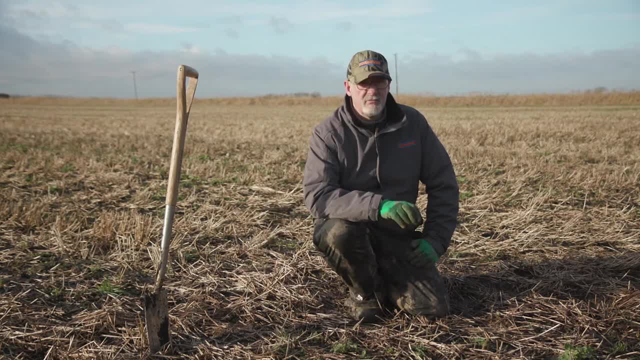 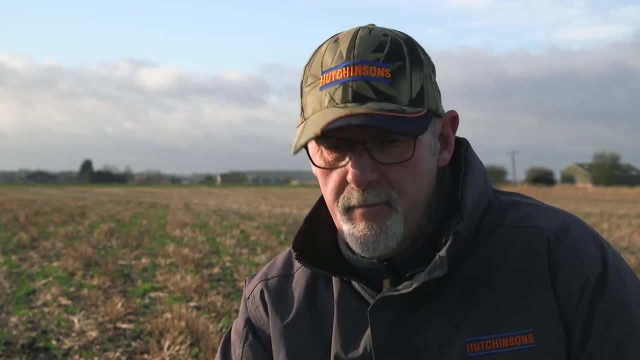 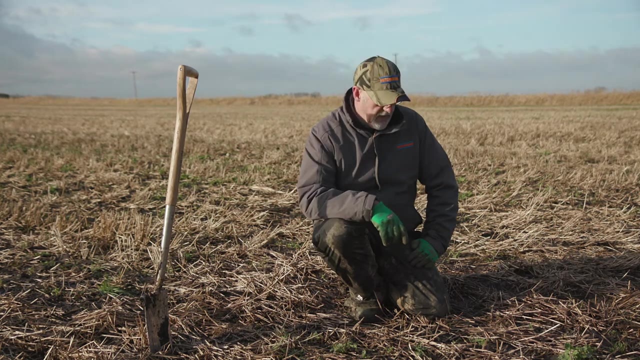 soils to give us really good drainage to depth and root penetration to depth. we needed to put their food on the surface. that's where they like to feed. So we just want to have a quick look now at what we can actually see has changed within the last four years and takes a little bit getting. 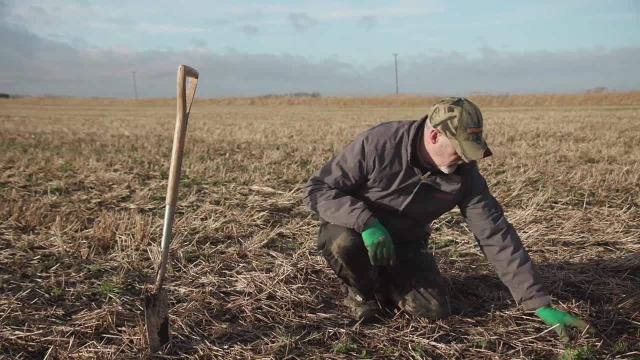 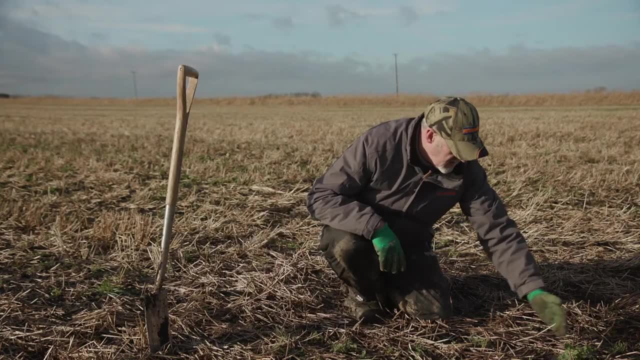 your eye in. but once you've got your eye in, you can start to see these little wigwams. they get formed on the surface of the soil and around each of these wigwams when you've got quite a thick layer of crop residue, like we have in this situation. so this is chopped up. 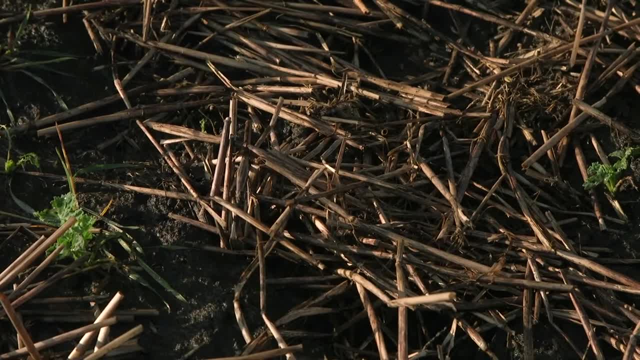 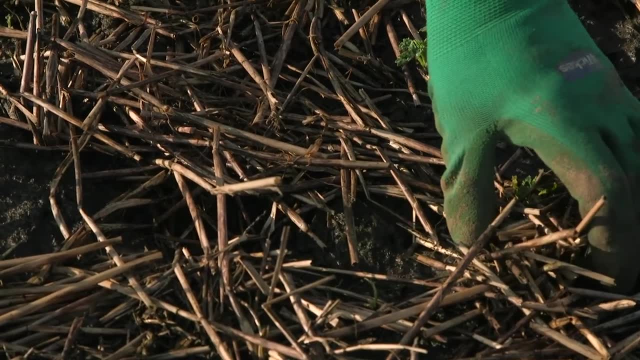 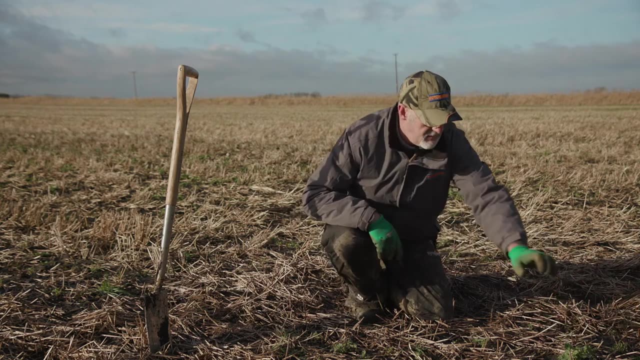 spring barley straw, but you can see this clear gap or area of bare ground surrounding this wig, this unnatural looking wigwam of straw. it's clearly been brought together and that's being brought together by an anisic worm, and we can count these middens within a square meter and 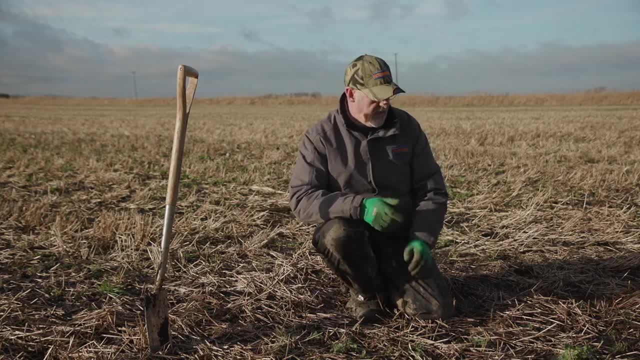 having counted them in here, you know we're now up to in four years. we've gone from nothing to about fifteen anisic worms per square meter. that's a really useful population, Because they can now come together and start to mate on a regular basis, lay lots of eggs and the 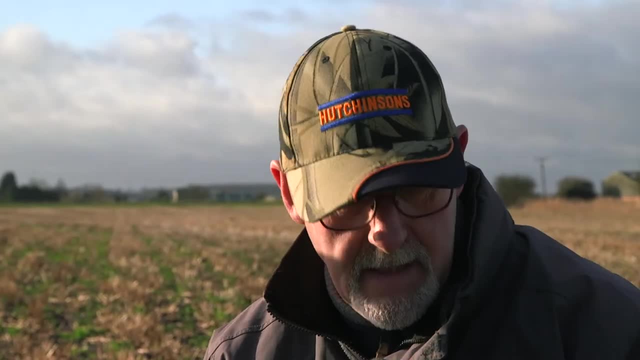 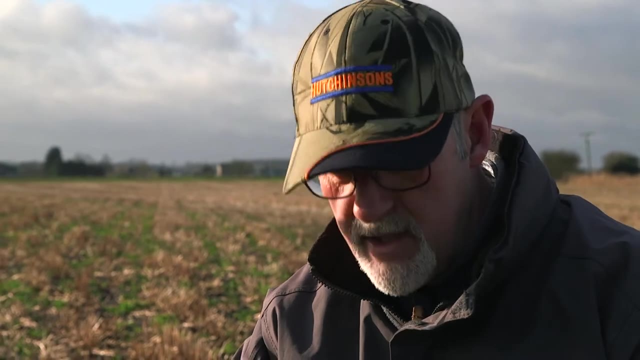 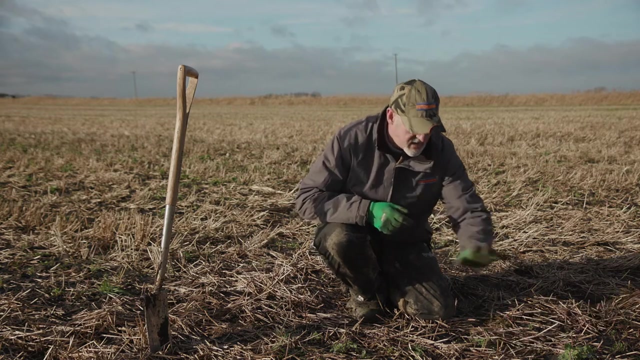 worm population really starts to expand very, very quickly. but when we're trying to build populations like this, we must remember that their food source must be placed on the on the surface. They're a key part of managing our residue. so place the residue on the surface as the 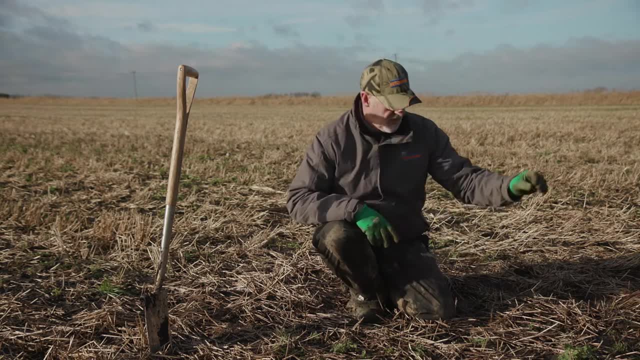 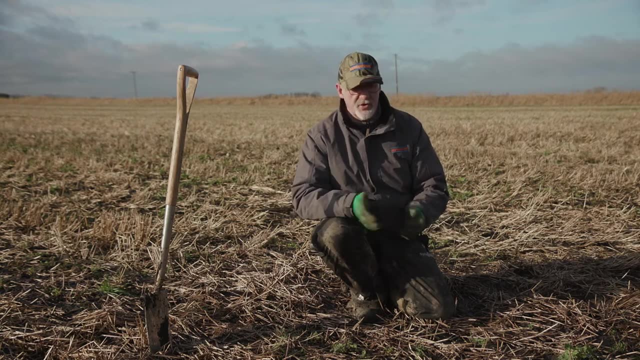 population builds, they will clear that surface of residue, take it down into the soil and then, taking that residue down into the soil, they then share that food source with endogenic worms which are living in the top 12 inches of soil or so, moving backwards and forwards or side to side in a horizontal manner, and they're the worms that really help. 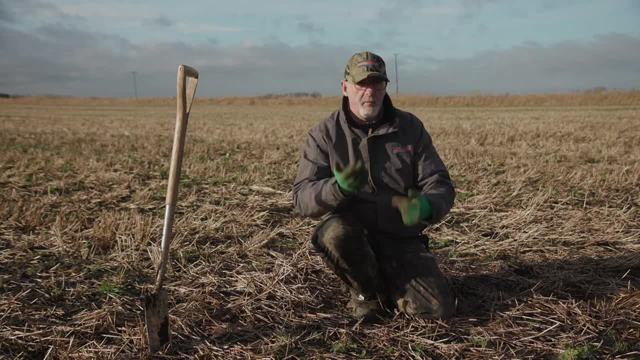 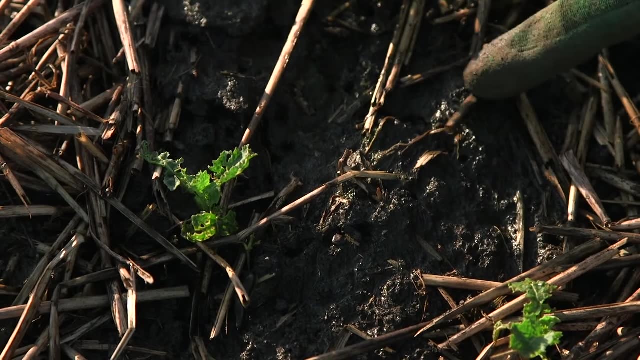 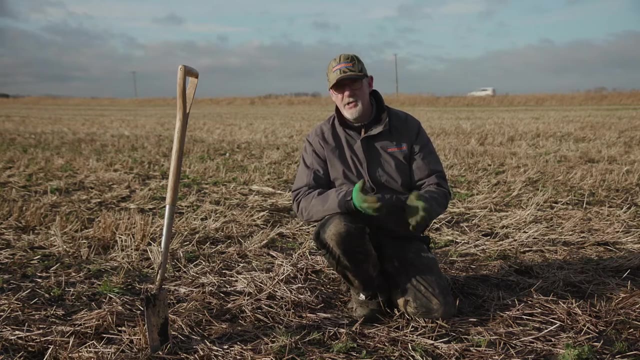 aggregate our soil and they're always popping in and out of the surface of the soil as well. you'll get lots of little holes popping up in the surface and you'll see lots of worm casts on the surface as well. that's all driven by epigeic worms. 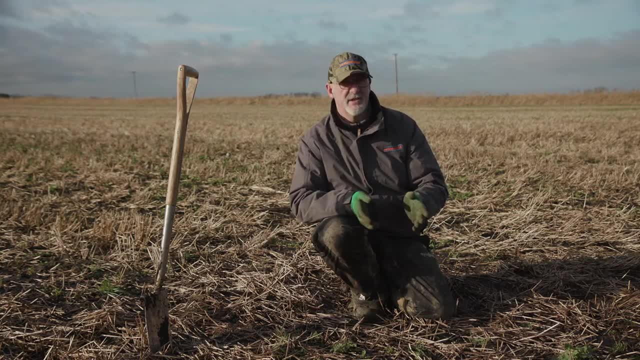 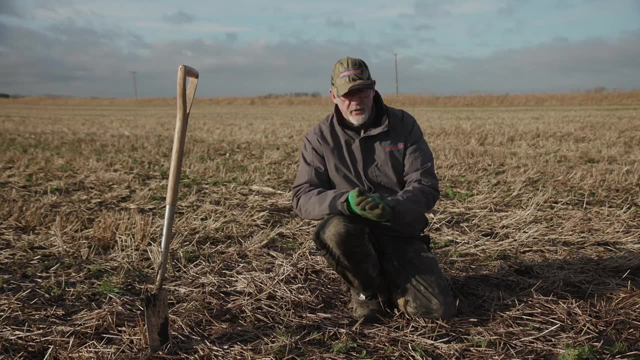 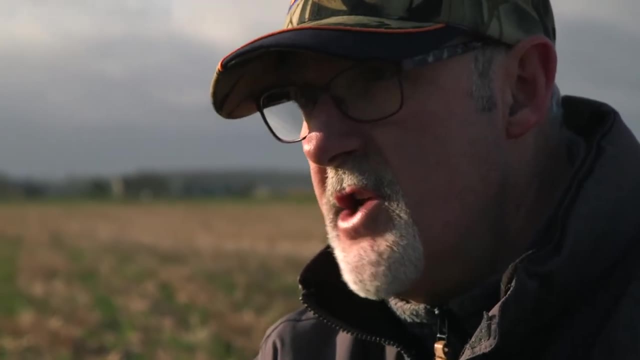 which are far less cultivation sensitive, because if we cultivate the soil and move it around a little bit, we just move those worms around a little bit as well. if we actually plow- let's say we plow 12 inches- we take all the worms within that 12 inches and just turn them over. so a large proportion of 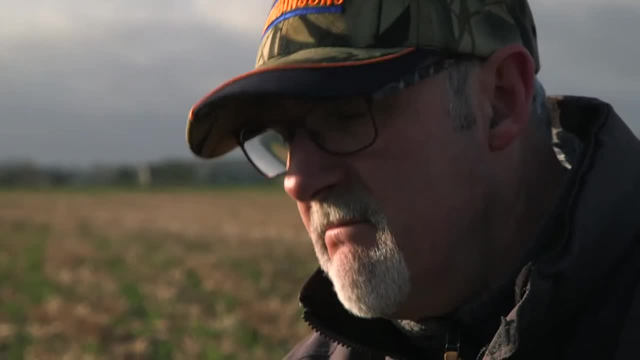 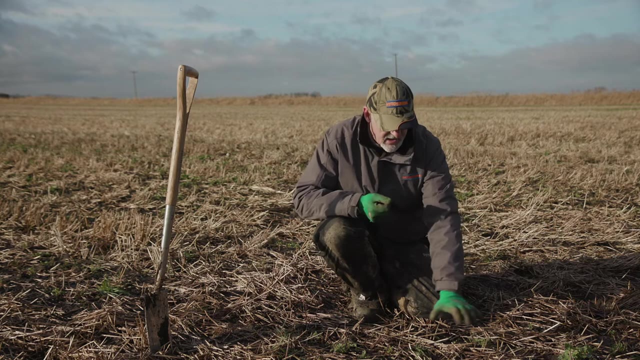 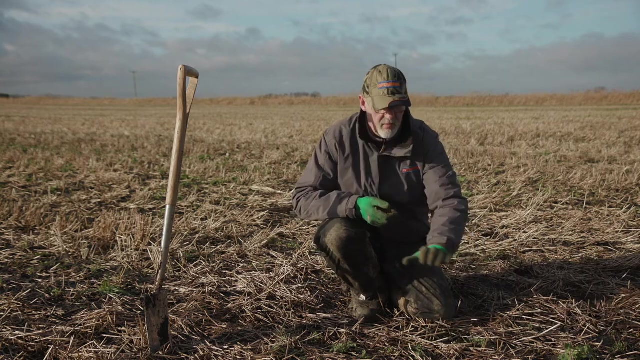 them again survive. They don't live in permanent burrows, so they just get on with the job. we'll always find epigeic worms in most arable soils. however, these anisic worms, these are the big deep working worms. they live in permanent burrows, so each one of these worm middens is indicative of an individual worm. 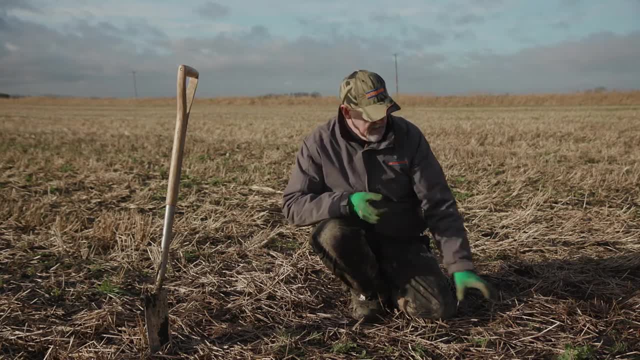 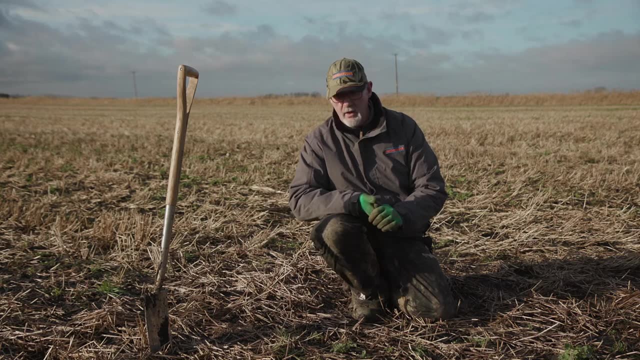 working in a burrow that can go two meters deep in the soil, and we don't have to get a spade out at all to ascertain how many worms per square meter we've got. We can just count these middens and have a pretty good idea of how our worm population is developing. 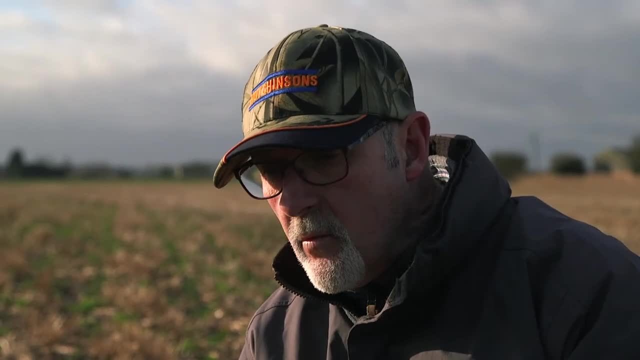 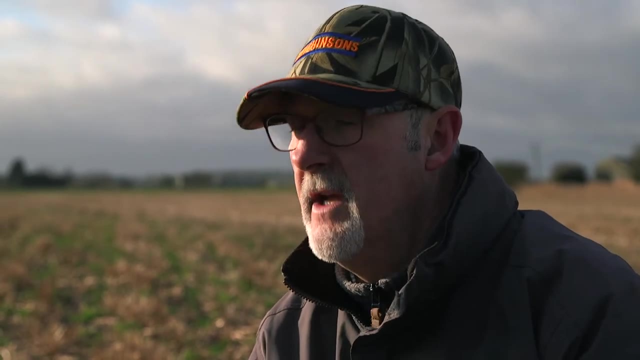 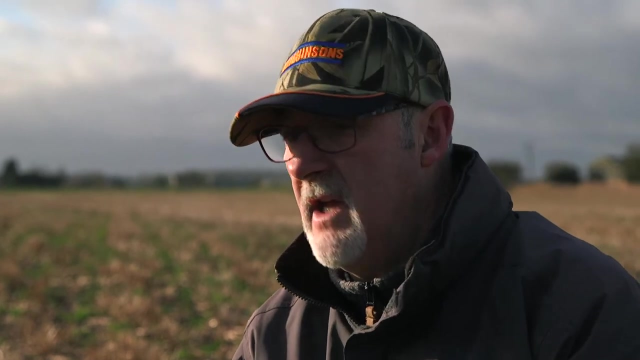 and that's happening really well here. we can see that because the way water is being managed through this soil as well is fundamentally changed in the last four years from from wet soil with ponding on the surface to after this year we've got no water ponding anywhere on any. 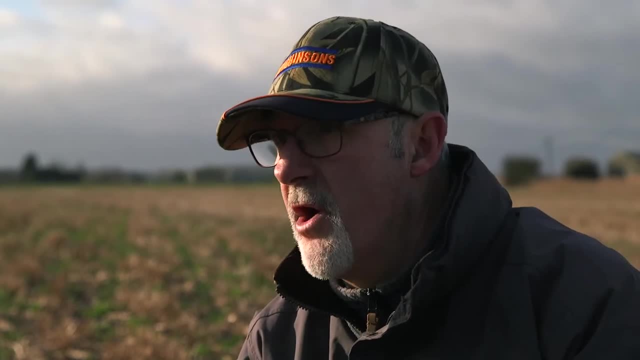 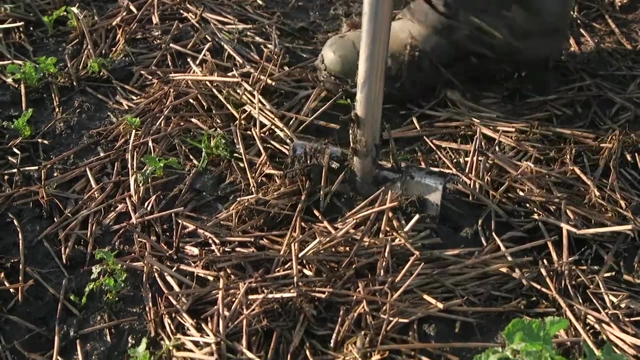 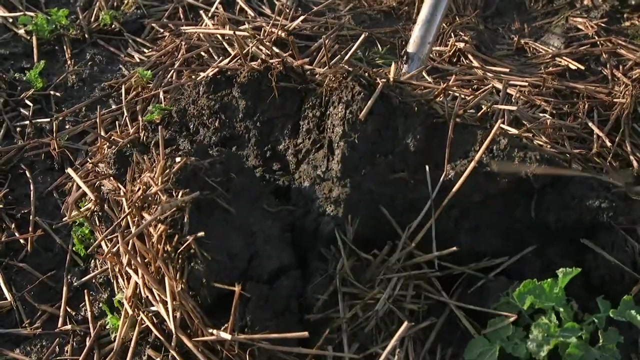 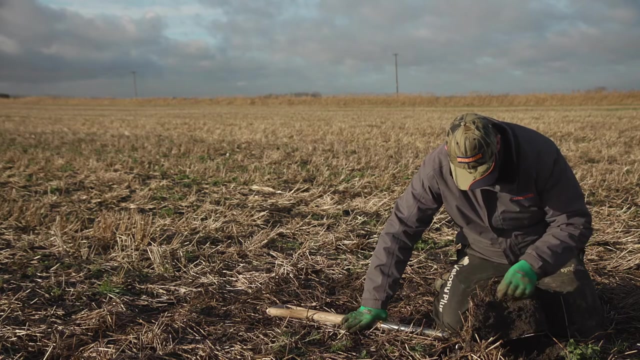 soil and good water penetration down through the soil profile, as George showed you and mentioned in the in the pit he was inspecting. So, having dug this area out here, with three worm middens on the, on the top of it we can start to see these permanent burrows with organic matter being drawn to the soil. 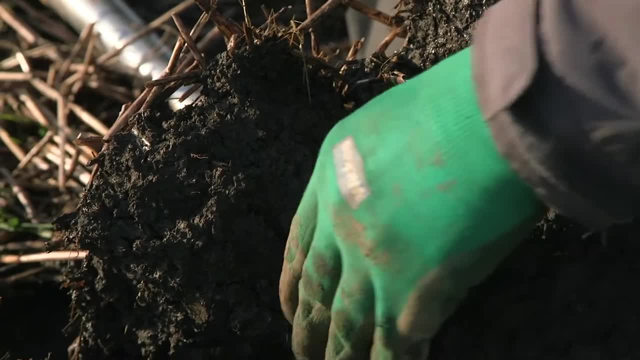 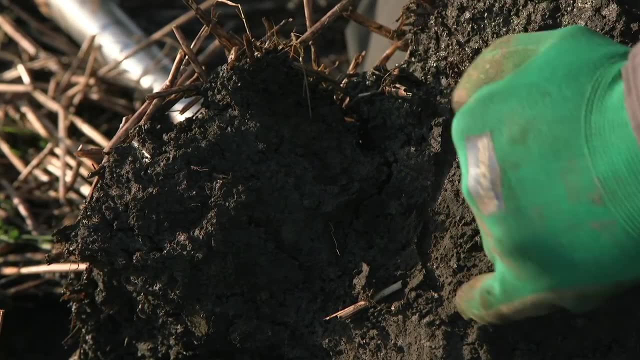 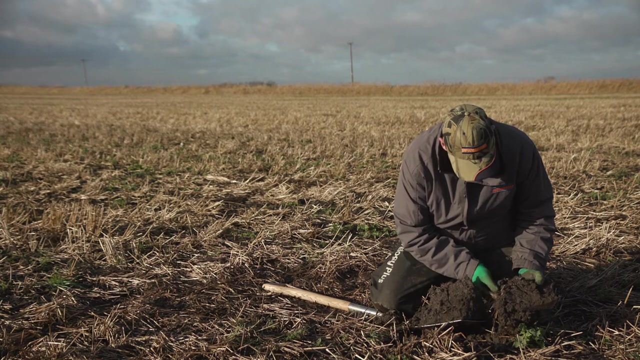 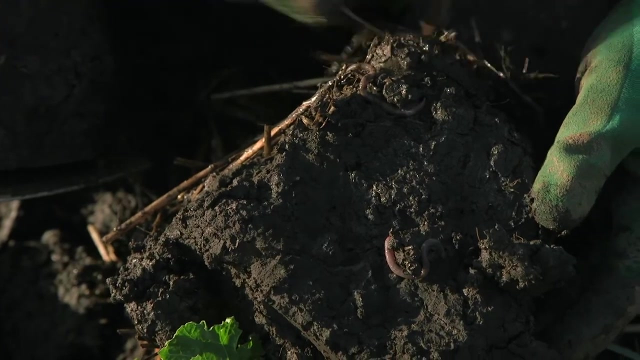 Being drawn down down into them and see them extend right down through the soil and that's giving us really good drainage and root access to to two depths. Good worm population starting to build in here. these are, in fact, our- I think, our- endogenic worms. good population now growing in here. some of these will be juvenile anisic worms. 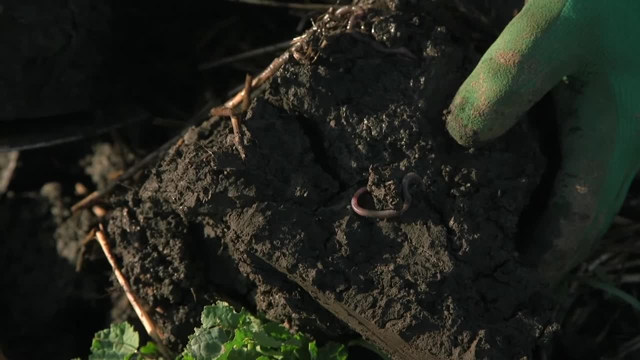 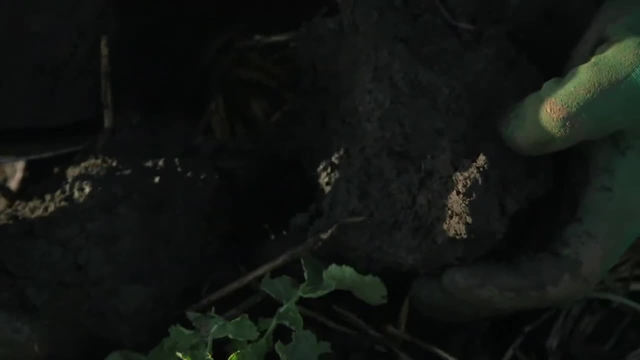 You can tell whether they're juvenile because they won't have a collar on and they tend to have quite a flat spade on the back of their tail and you can start to see the different colors that we get. and that's typical of these endogeic worms is we get all sorts of colors: yellow ones, gray, 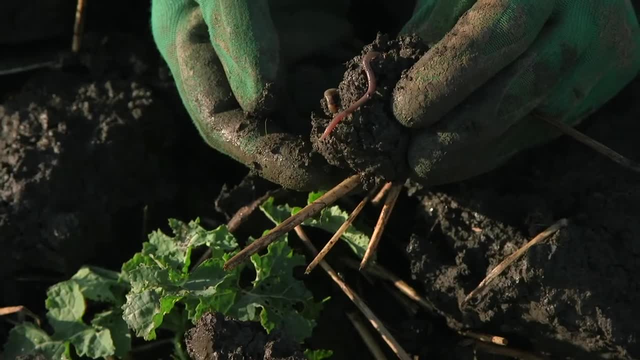 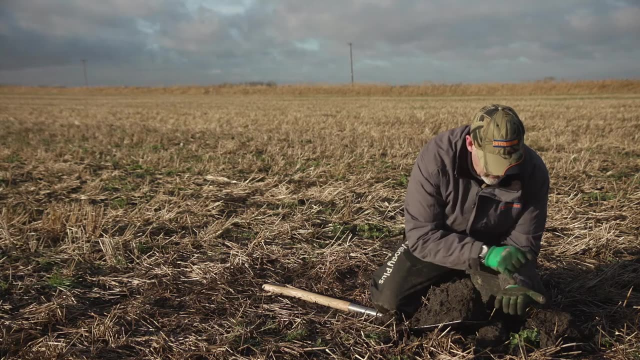 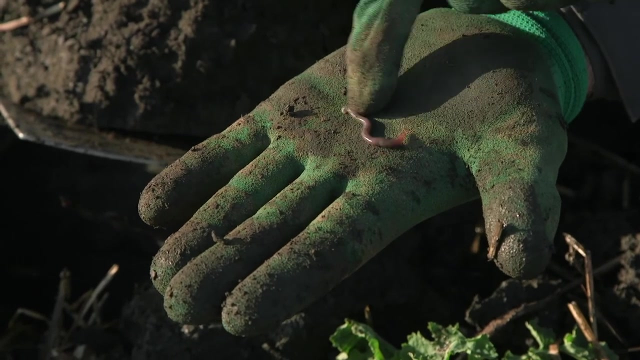 ones, green ones, one of the other things that happens if it's an endogeic worm. when you put it on your your hand they tend to curl up in a little ball. this one is a juvenile anisic worm. it's got a slightly flat tail. he just looks right. he's not curling up in a little ball. 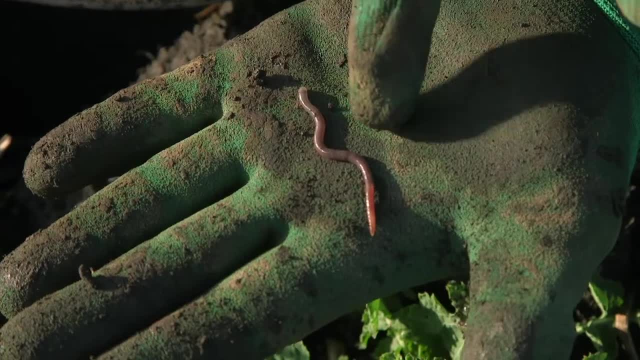 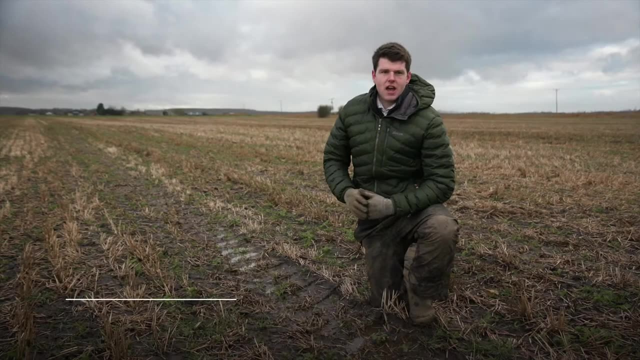 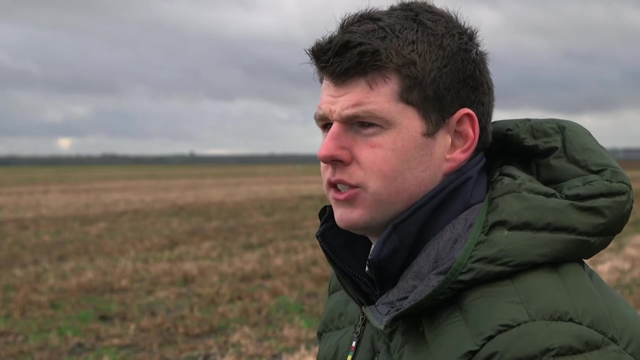 on my hand he's looking for his get out route and there's no collar. so that is definitely a juvenile worm, most likely an anisic. One of the main concerns I have from growers when adopting a surface tillage type approach is: what am I going to do with my tram lines and 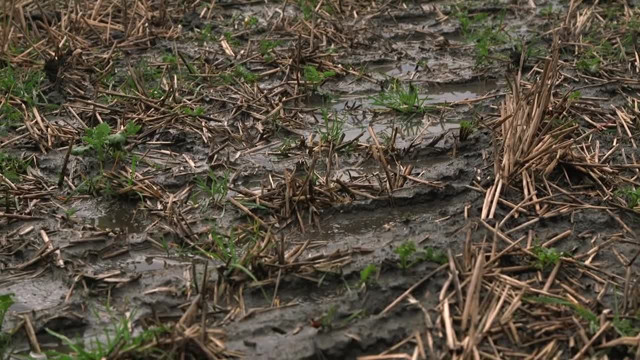 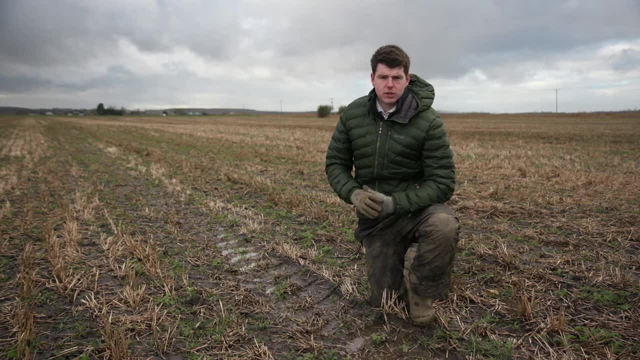 harvest wheelings? and my simple answer to that would be: looking at this field, what harvest tram lines and wheelings? This system builds much more resilience into the soil and, as you can see in this field, which has been trafficked several times on what has been quite a tricky Autumn, the compaction or the depth.